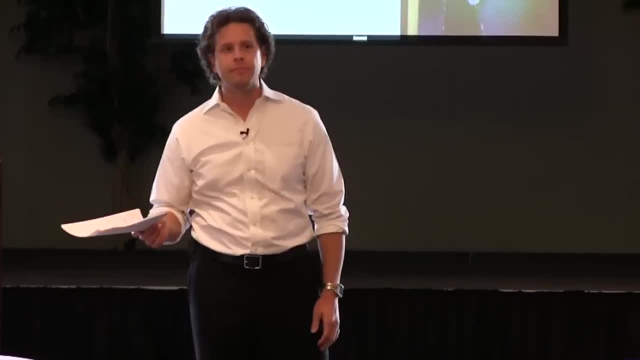 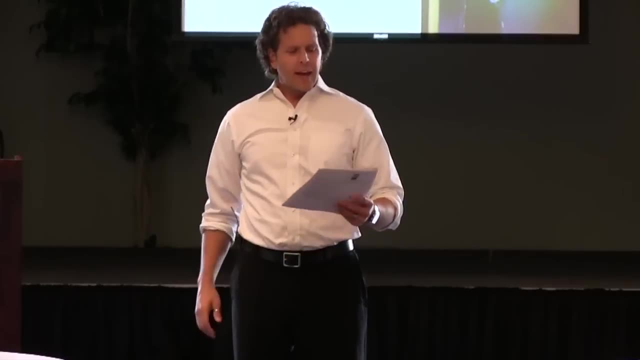 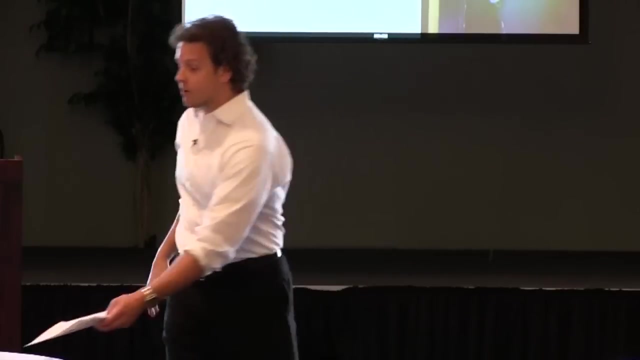 An exact quote from one of my clients. This is a man who is very intelligent, one of the best at what he does, And he said to me: Jason, I want to hire you so that you can help me conquer my fear. I actually gave a presentation to about 160 people and he comes up to me afterwards and he says: that's all great stuff, but here's the thing. 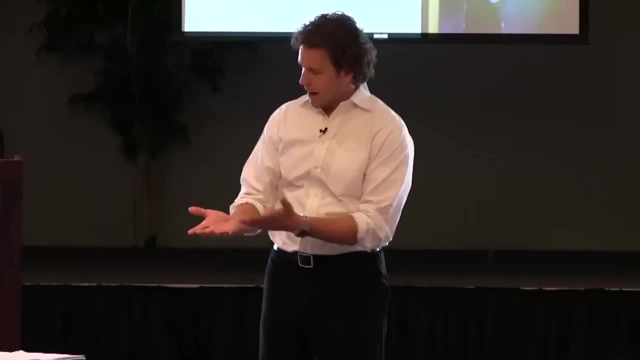 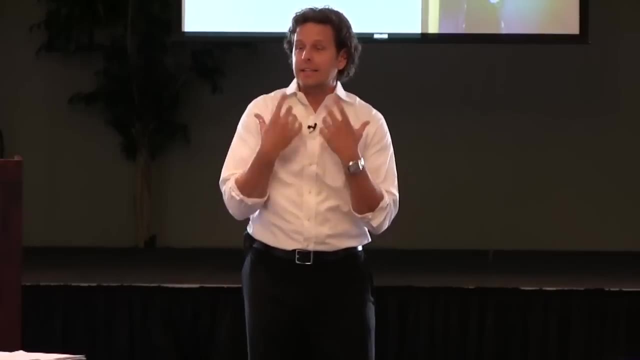 I have such an irrational fear that my hands they sweat and I forget what I said when I presented. And I'm so scared when I come up front that I he says I can't. I don't even remember what I'm going to say. 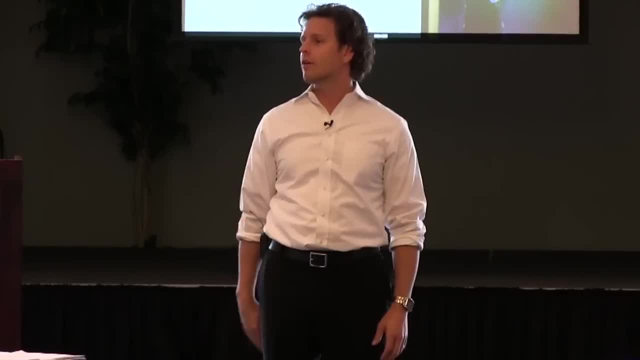 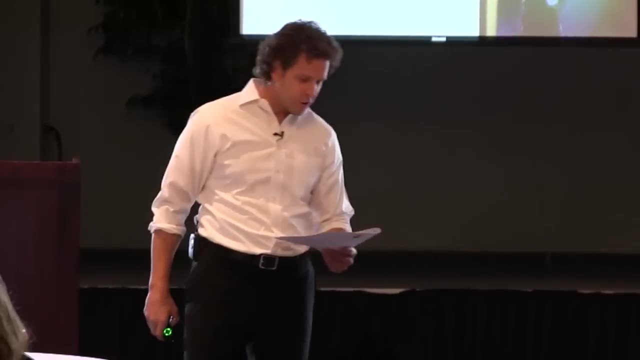 Even though I practiced. what should I do? I said: set up three two-hour sessions with me and we'll fix it. And here's what he said. afterwards I sent him an email and I said: did you conquer your fear in this last presentation? 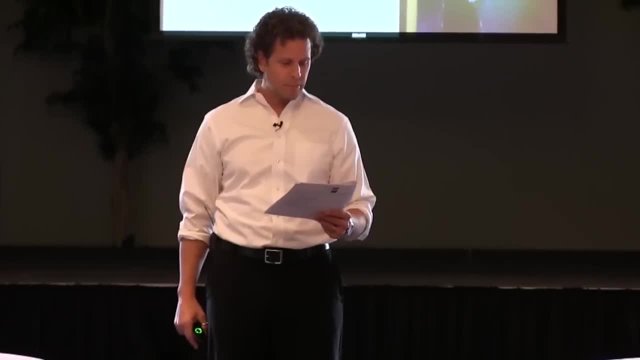 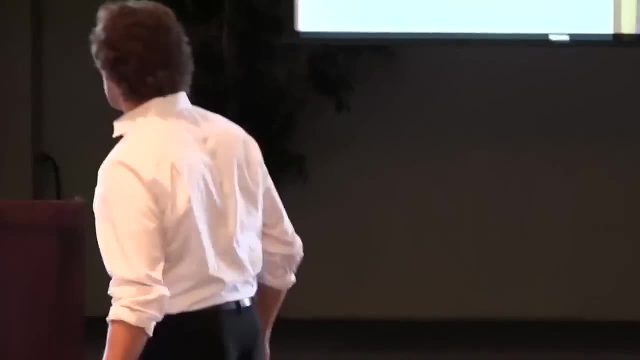 Here's what he said. The short answer is yes. I was able to give my presentation effectively In front of a crowd without the security of a podium or table, Because when you go behind a podium, when you go back here, you lose your body language. 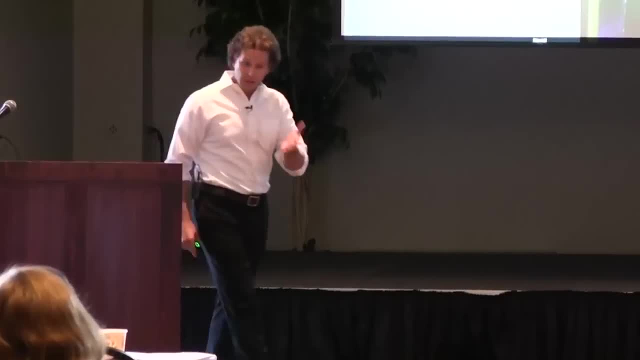 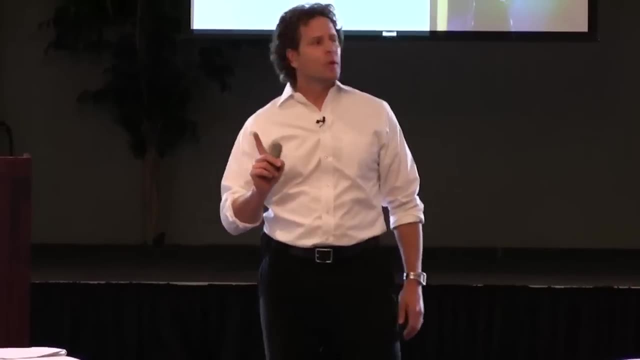 It's gone. All you have is your facial expressions and your tone, But when you're here, you've got body language again, which, remember, is what percent? 55. So what did I do with this guy? I did these three things. 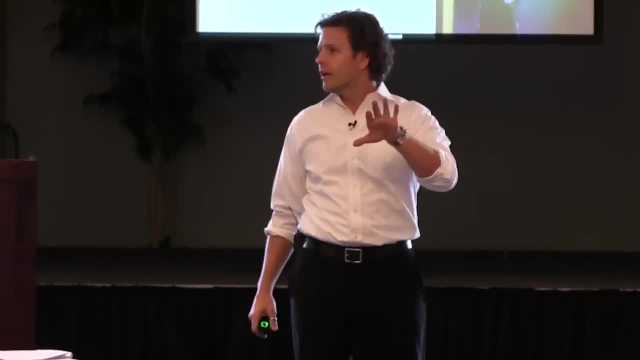 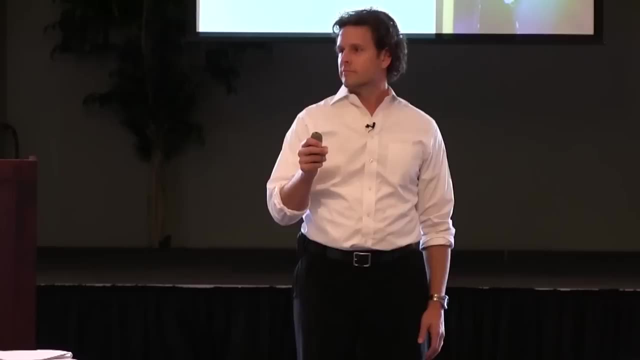 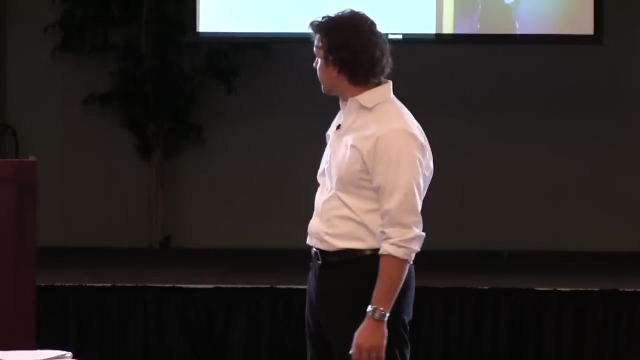 The first thing I said to him- and this is something you're all going to want to write down, because it's so safe to hear this: It's not whether you're nervous, It's whether you show, it, Isn't that interesting? He said: well, what does that mean, Jason? And I showed him this slide. 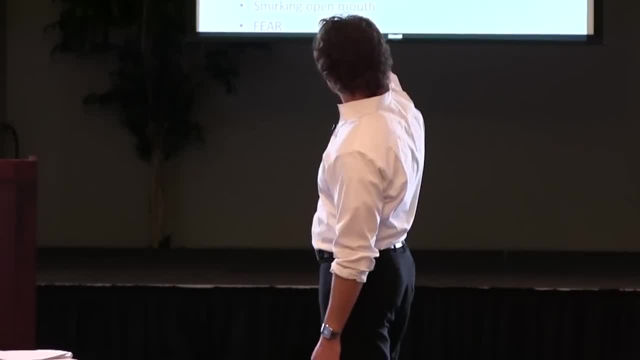 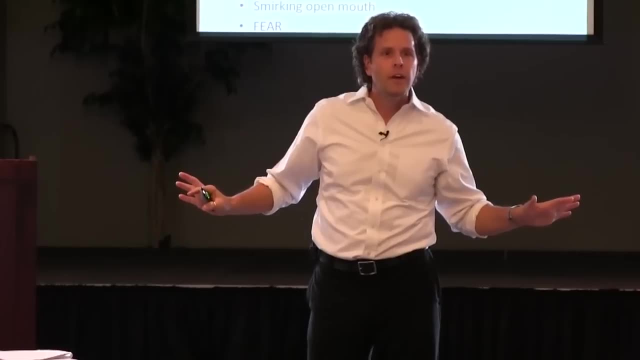 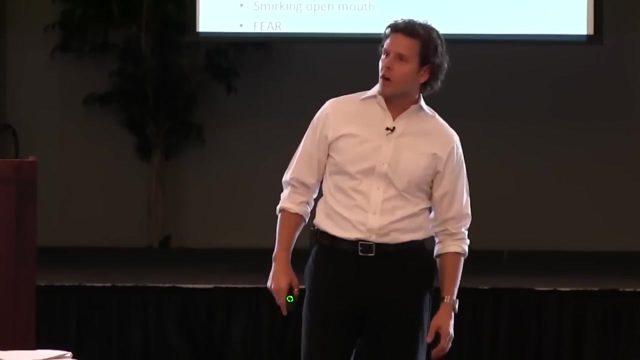 Stop doing these things. These are the top 12 things that, if you do them, you look nervous, And when you do it, your audience doesn't feel what Safe. Check this out. Shifting weight: How many times have you seen people shift their weight back and forth like this? 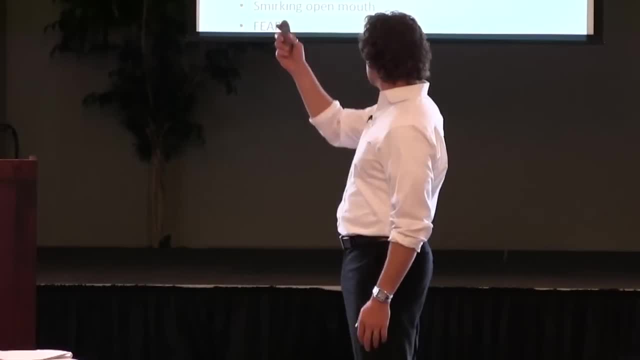 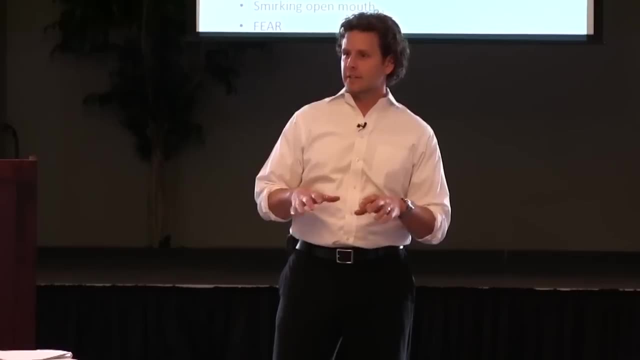 Or rubbing their collar, or rubbing their arms, overusing the mouse in a demo, blinking, excessively, widening eyes. Here's one of my favorites: The T-Rex stance. You guys ever seen this with presenters? Why do they do this? 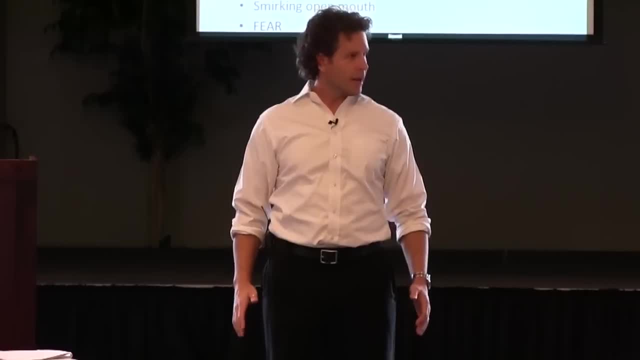 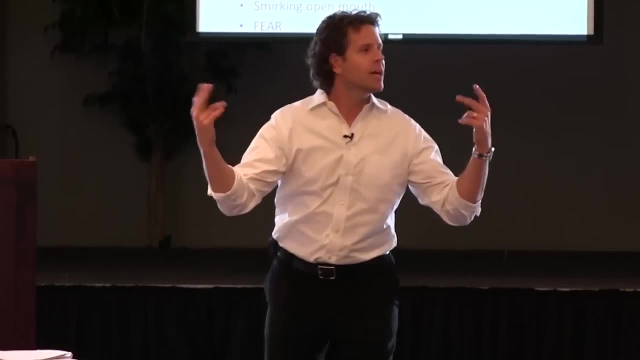 Because, you should know, this is the most calm, comfortable stance on the planet, where your hands are to your sides, feet are standing still like a magnet and your head's just moving back and forth like a swivel, looking at people. Because what are you looking at when you're looking at me right now?